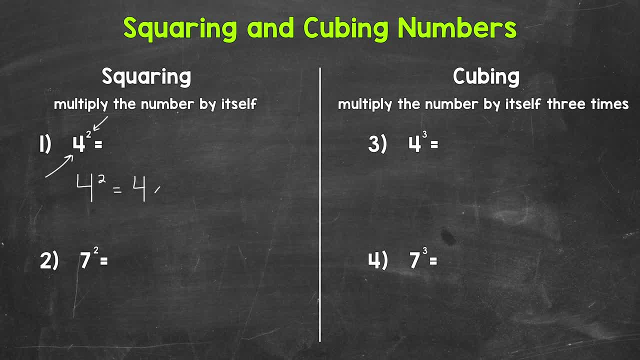 So four squared equals four times four. We take that base of four and expand it out two times Four times four, that equals sixteen. So four squared equals sixteen, And it's as simple as that. Now, a common mistake when working with exponents is to multiply the base by the exponent. 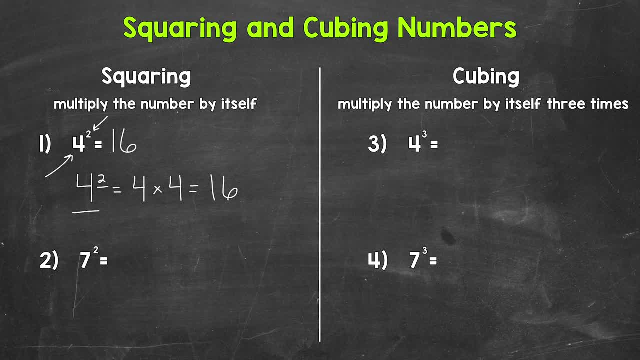 For example, in number one, four times two would equal eight and would be incorrect. So again, don't multiply the base by the exponent. Expand the base out however many times the exponent tells you. Before we move on to number two, I do want to mention why we call it squaring a number. 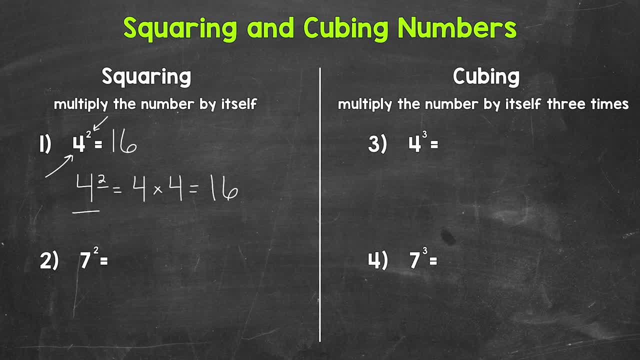 If we take a look at the number, we can see that number squared equals eight. If we take a look at a square, we can see why we call it squaring a number. For example, if we were to take a look at a square with side lengths of four, 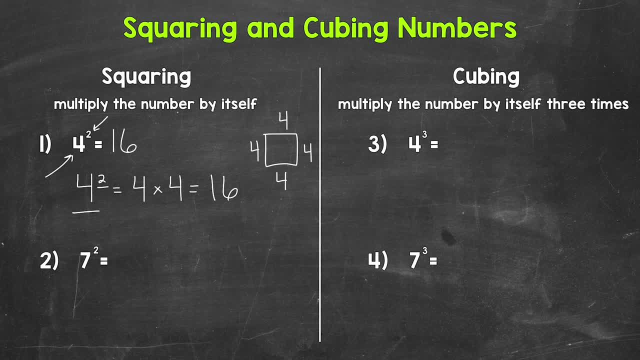 we can find the area of this square by doing four times four, or four squared, That gives us an area of sixteen. We can square a side length to find the area of a square. We can square a side length to find the area of a square. 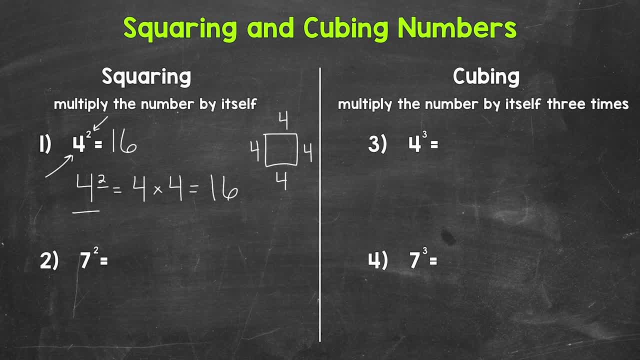 We can square a side length to find the area of a square. So you can see the relationship between squaring a number and the area of a square. Squaring a number or squaring a side length gives us the area of a square. Let's move on to number two, where we have seven squared. 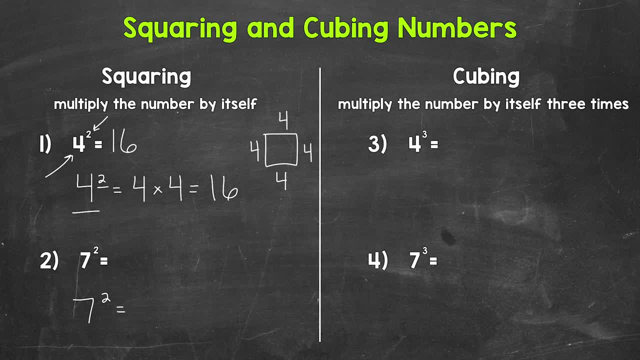 Now, seven squared that equals or means seven times seven. Expand that base of seven out: Seven times seven equals forty-nine. So seven squared equals forty-nine. That's how we square a number. Let's move on to cubing a number. 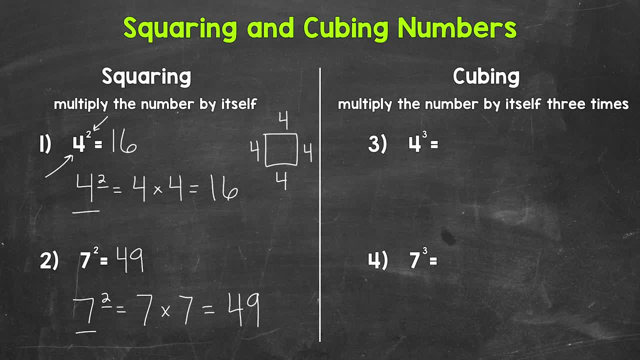 Starting with number three, where we have four cubed. So anytime we have an exponent of three we are cubing a number. Now again, when working with exponents, the bigger number to the left is called the base. So this four is the base for number three. 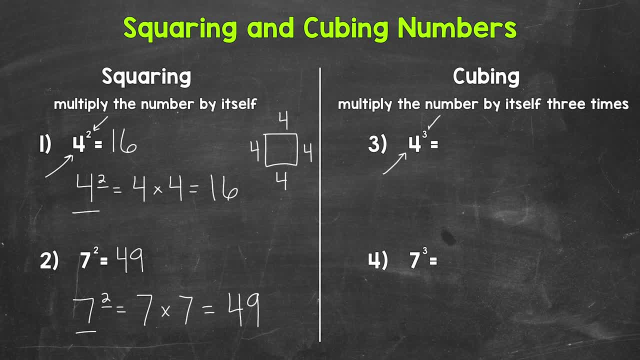 The smaller number to the right is called the exponent. So this three is the exponent for number three. That three tells us to expand the base out three times and multiply that number by itself three times. Let me rewrite four cubed down below here. 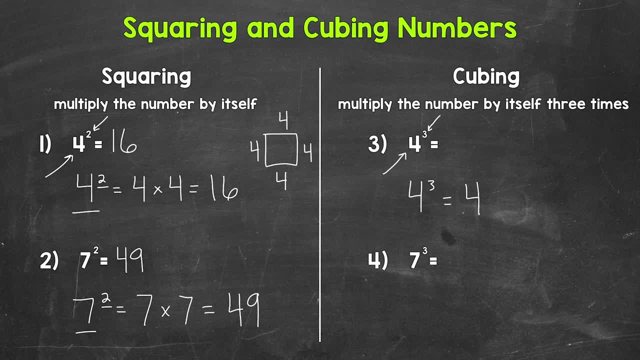 So four cubed means, or equals four times four. So four cubed means, or equals four times four. Take the base of four and expand it out three times Four times four equals sixteen times four equals sixty-four. Four cubed equals sixty-four. 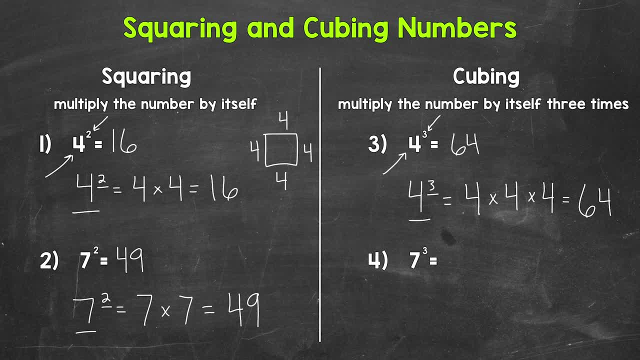 Now again, avoid the mistake of multiplying the base by the exponent. So for number three, four times three would give us twelve, And that would be incorrect. Expand that base out however many times the exponent tells you. Before moving on to number four, I do want to mention why we call it cubing a number. 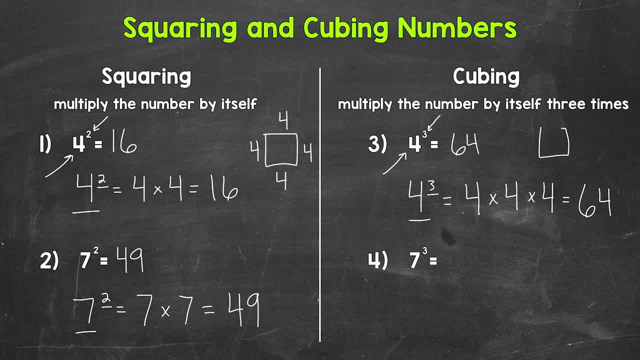 So let's take a look at a cube. For example, if we were to take a look at a cube with edge lengths of four, we can find the volume of this cube by doing length times length. We can also find the volume of this cube by doing length times width times height. 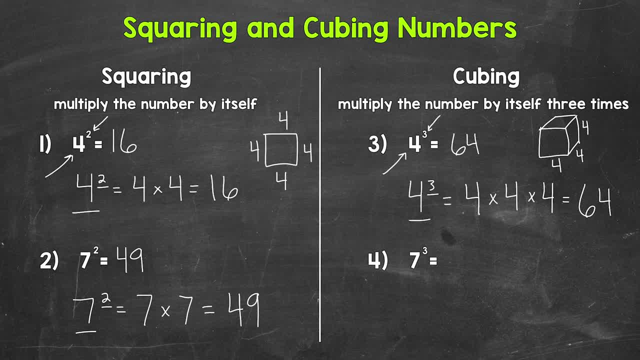 which would be four times four times four, which is just four cubed. We can cube an edge length to find the volume of a cube. So you can see the relationship between cubing a number and the volume of a cube. Cubing a number or cubing an edge length gives us the volume of a cube. 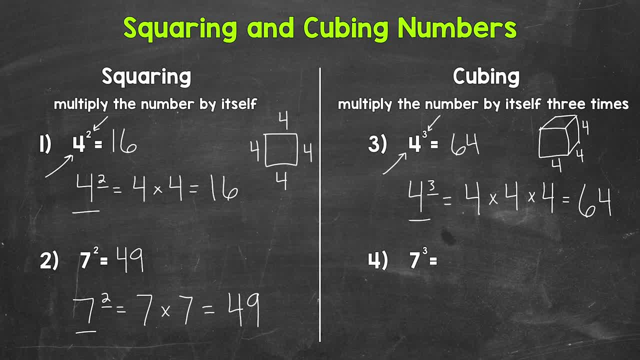 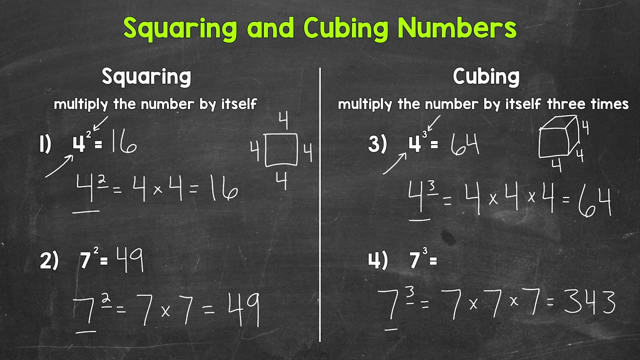 Let's move on to number four, where we have seven cubed. Now, seven cubed equals, or means seven times seven times seven. Expand that base of seven out three times Seven times seven is forty-nine times seven equals three hundred forty-three. So seven cubed equals three hundred forty-three.